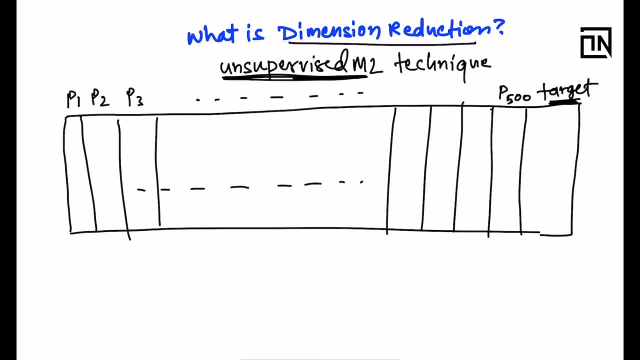 into picture when you do dimension reduction. So over here, the problem which you will face in using this data to fit your machine learning models is you need to take into account all the 500 columns, okay, and when you take 500 columns into account, this kind of data or more, 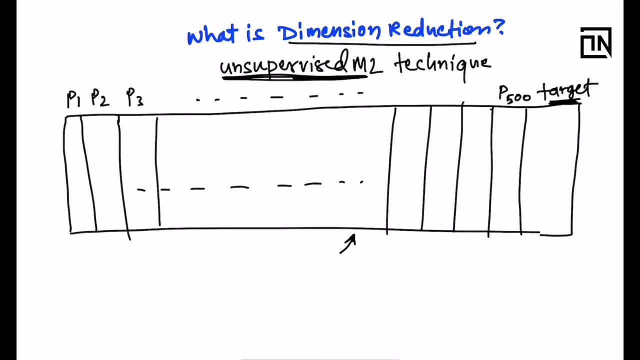 let's say you have 1000 columns or 2000 columns. these kind of scenarios are very common in text mining. so so whenever you are doing natural language processing, you are trying to create a model, let's say, for ticket classification. so the ticket description data needs to be converted. 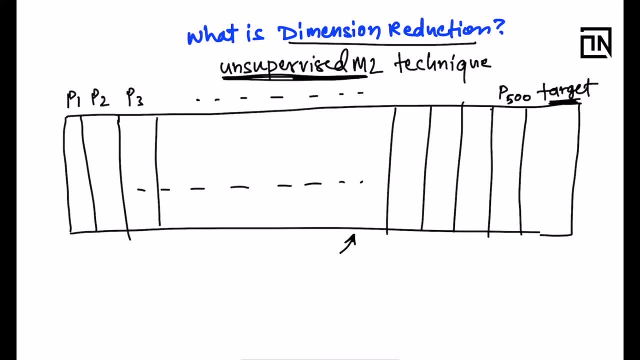 into numeric form and then each word will represent one column, also known as the document term matrix. in such kind of data sets, 1000 columns or 2000 columns of predictors is very common. so in such scenarios, let's say, if you use that data to try to fit through a machine learning, 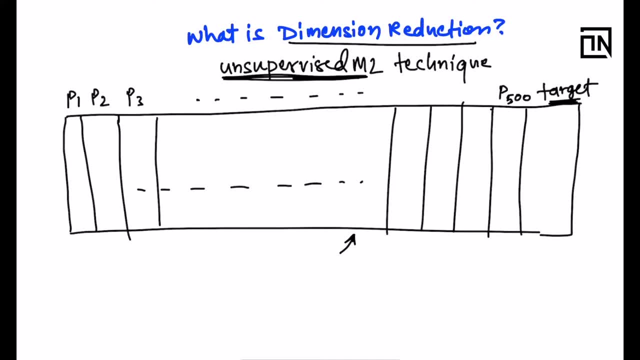 algorithm. it will take large amount of time and it will be painfully slow. so what you can do is, instead of fitting these 500 columns into a data set, you can use a machine learning algorithm. instead of fitting these 500 columns into a data set, you can use a machine learning algorithm. 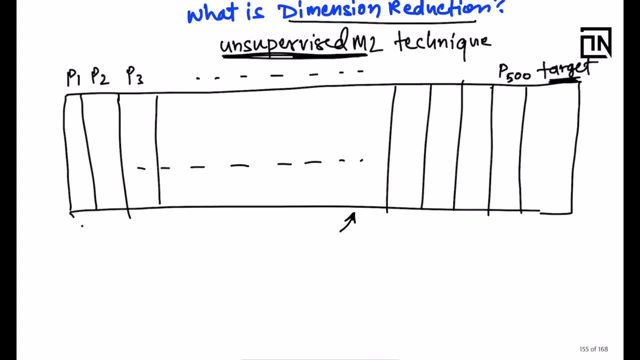 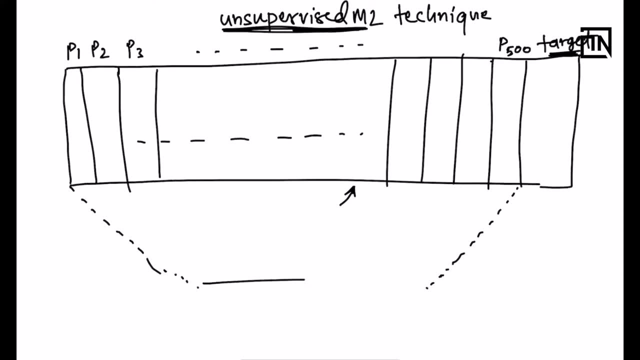 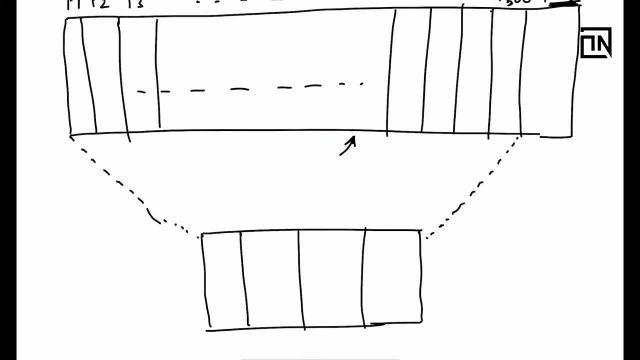 all together. is there a way in which you can shrink these 500 columns which you have, 500 predictors? i am shrinking the number of predictors only with some smaller number of columns. let's say, let me call these columns the very famous principal components, let's say principal. 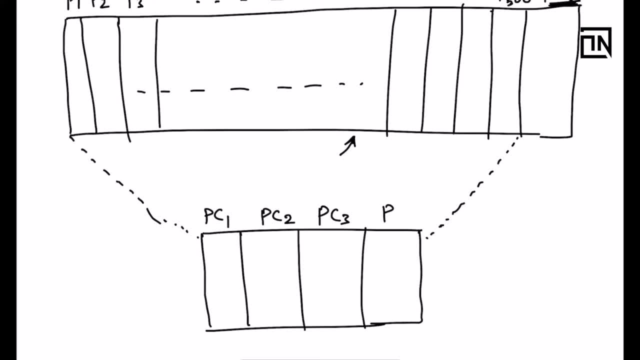 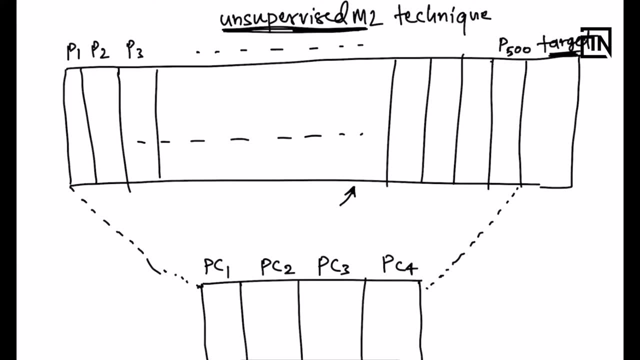 component one, principal component two, principal component three and principal component four. so i am representing these columns, these 500 columns with just four columns, or maybe thousand columns with four columns, or five columns, or ten columns. how do we decide these columns? it is based on the algorithm to algorithm. 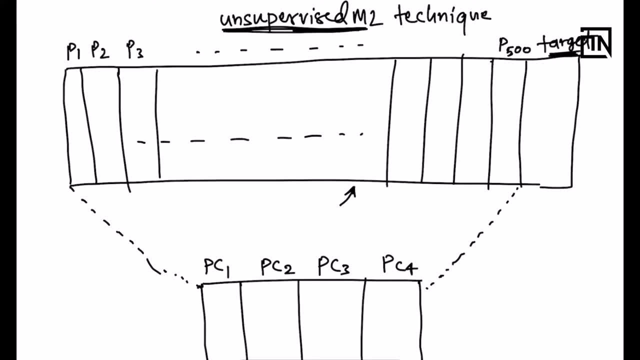 okay, so we will discuss that going further, but this is the overall idea. i am doing some work only on the predictors data, so i am shrinking the predictors representing large number of predictors with smaller number of predictors. how many predictors should i choose to represent these 500? 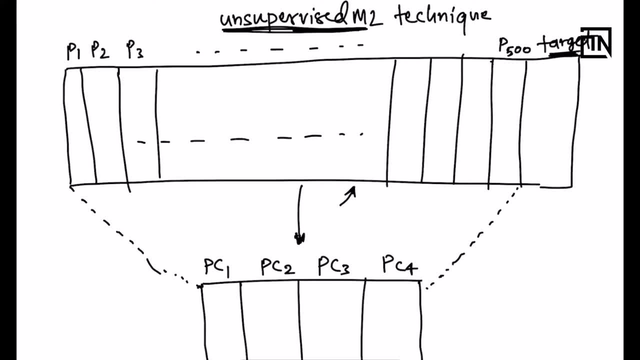 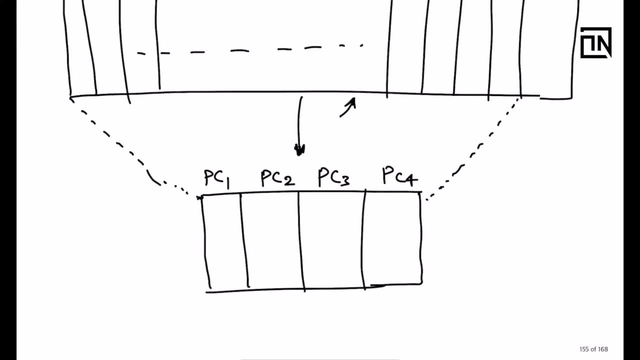 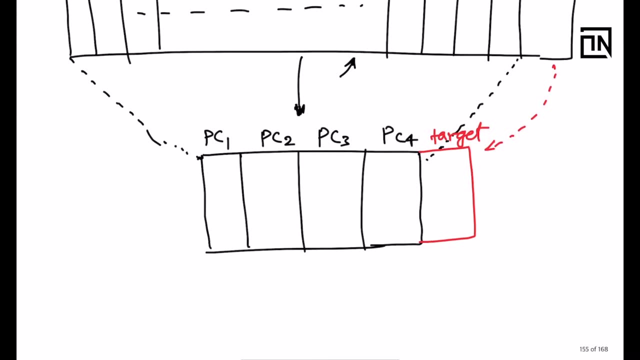 predictors. this is also something which varies from algorithm to algorithm, which we will discuss further. okay, so once i have given this representation of 500 columns, with just 400 columns, now i can bring in the target variable, create this new data. so now this new data is a. 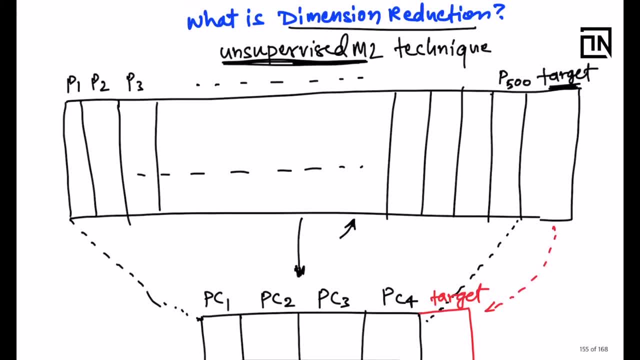 representation of the old data which was having high number of dimensions. dimension means what columns? so these are nothing but dimensions. every column represent one dimension. so these are nothing but dimensions. every column represent one dimension. so if there are so many dimensions in my data because of xyz reasons, i can somehow represent it. 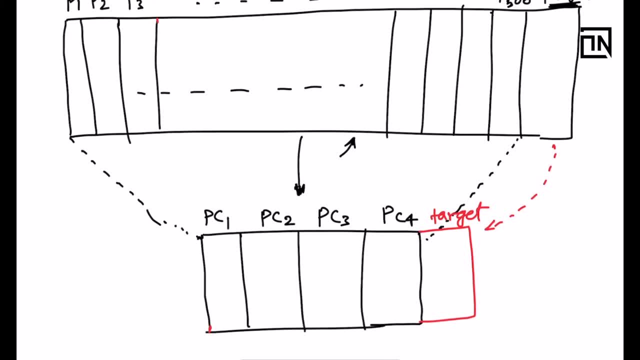 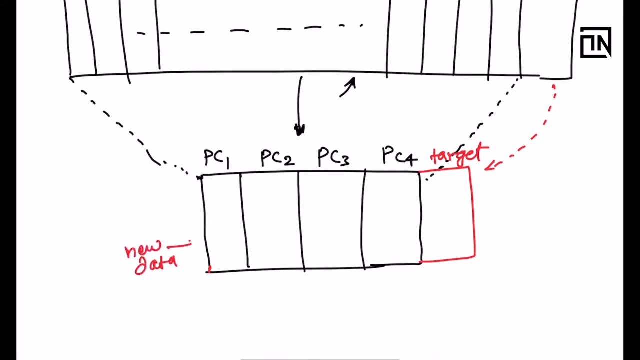 with smaller number of dimensions or smaller number of columns, and these dimensions could sometimes be called as factors and sometimes called as principal components, etc. so different algorithms will name it differently, the way they combine it. okay, so once you do this now, you have a new data and on this data you can fit your machine learning algorithms. 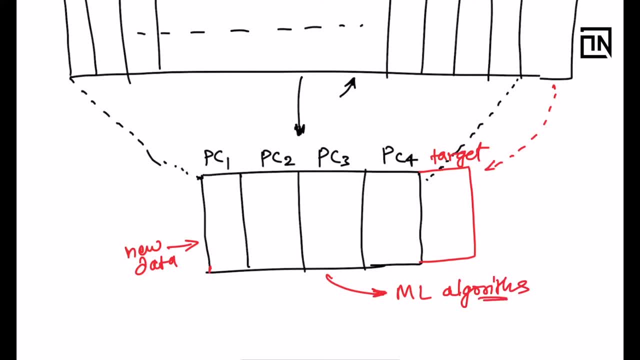 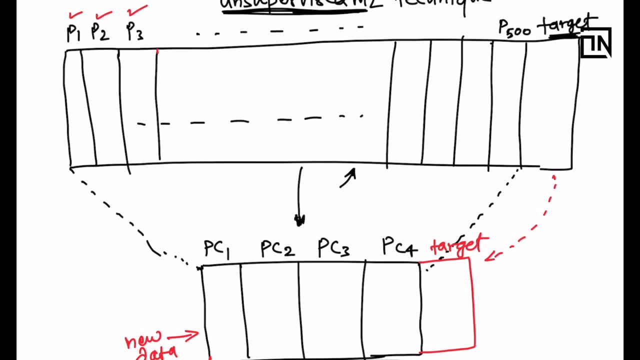 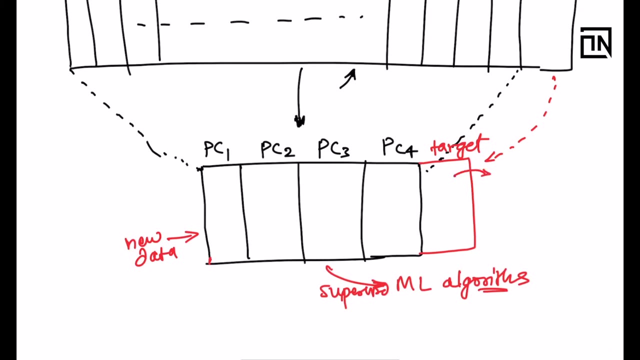 supervised machine learning algorithm because, let's say, the target variable is there, then definitely either you are doing regression or you are doing classification. so, whatever is the scenario, if you are trying to predict something, which is the number, then you will fit supervised regression machine learning, or if it is a class, then supervised classification machine. 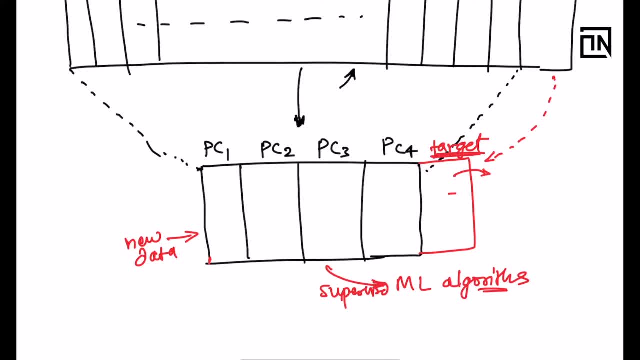 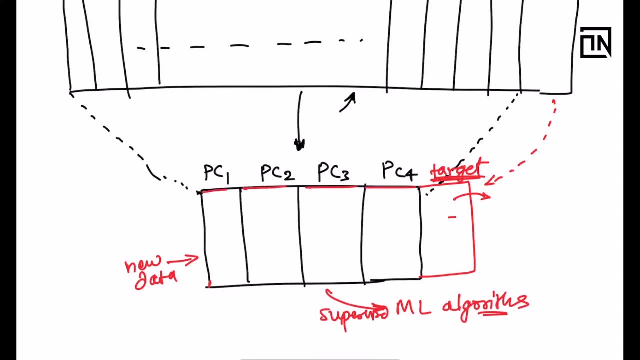 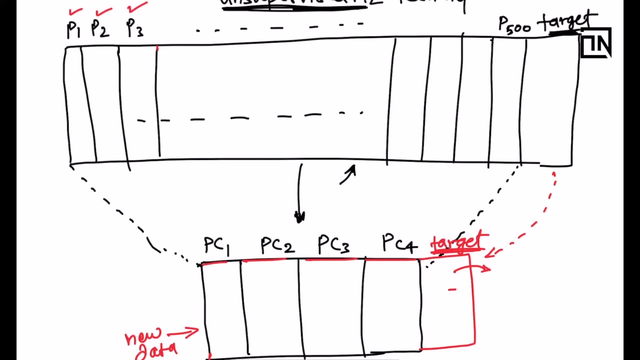 learning depending on the target variable. okay, but the crux is, your predictors are now shrinked to a smaller set of columns. okay, the whole journey of how these predictors are shrinked to smaller set of columns. this is something what we call as different. this is something 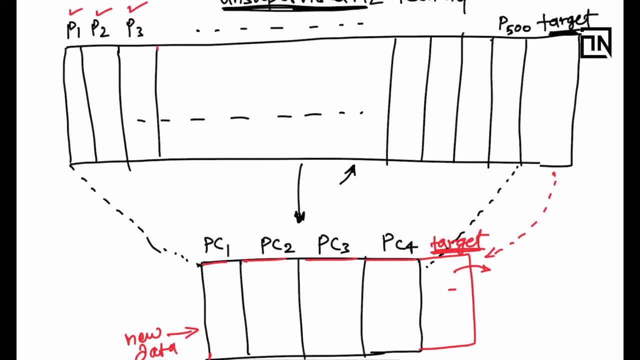 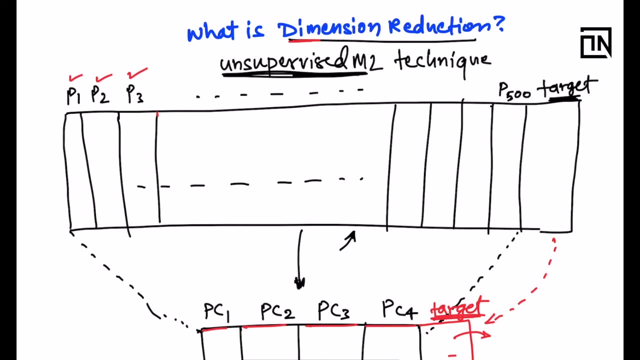 which is very different for different algorithm. for example, in factor analysis, it will happen differently. in principal component analysis, it's different, it will happen differently. or independent component analysis, it will happen differently, so on and so forth. so what is the need for dimension reduction? why do we require this activity to to be performed? because, if you choose, 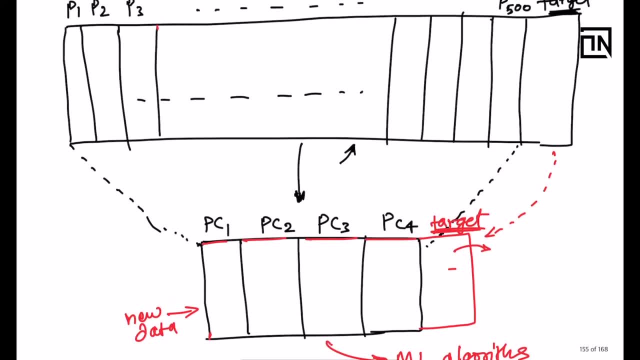 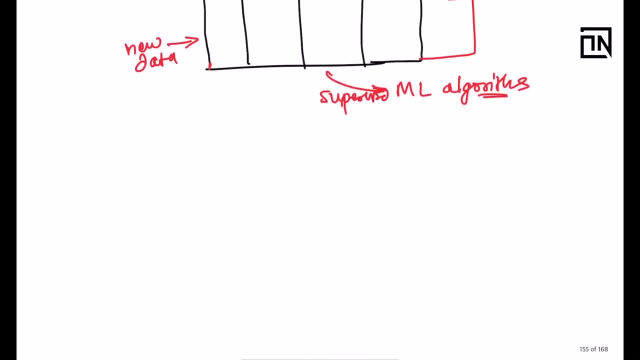 all the predictors, then your model training on this old data or the raw data, the model training, will be very slow. so if your data has high number of dimensions, high dimensionality, what we call- if your data is suffering from high dimensional, high dimensionality or too many, call too many. 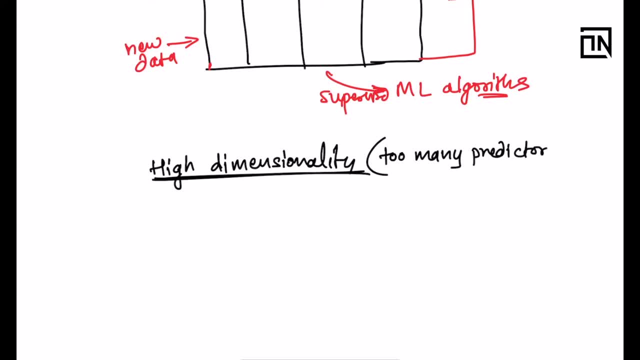 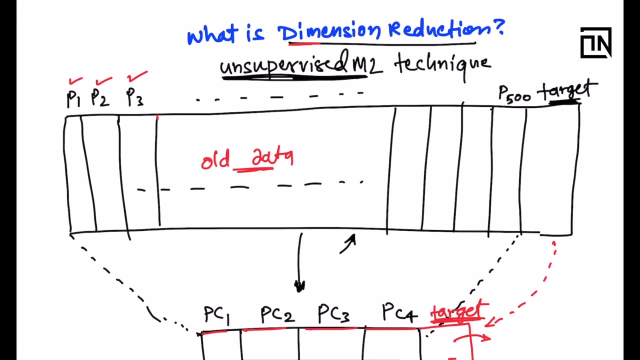 predictors, because target variable is always one. so, if this is the issue, what it will impact on your machine learning training is, first of all, it will be slow- and this is no brainer- if you have more columns in order to learn, more columns in order to find the best column out of it, or trying 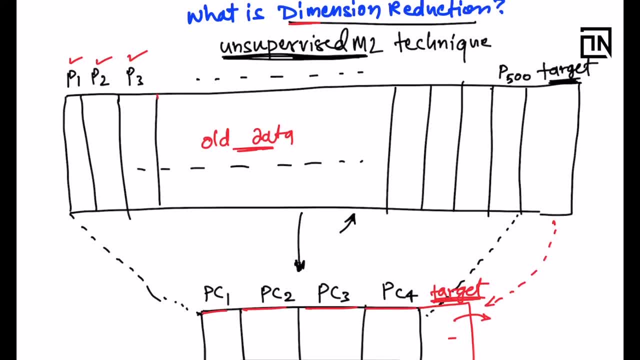 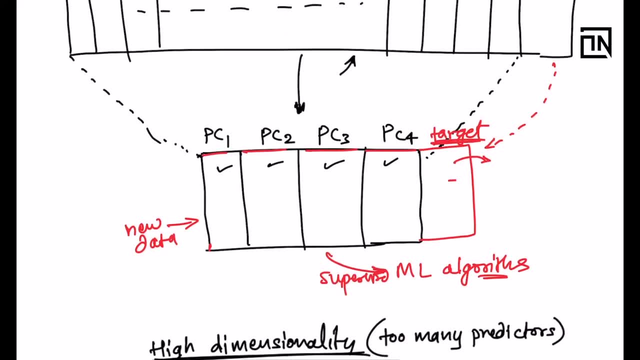 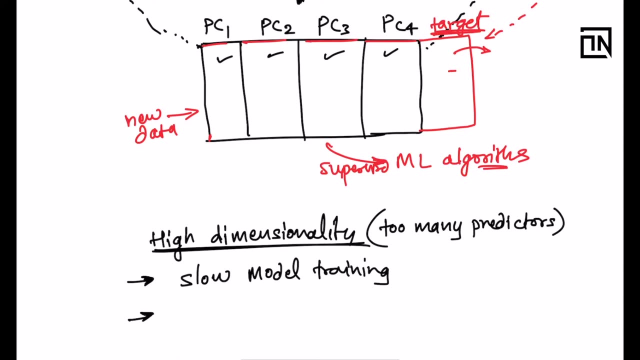 to find the equation of all the columns you will have, you will have to do more computations, and if you have less columns then you will have to do lesser computations. okay, and your algorithm will run fast. so once you convert your data into the reduced dimensions or a smaller version, or 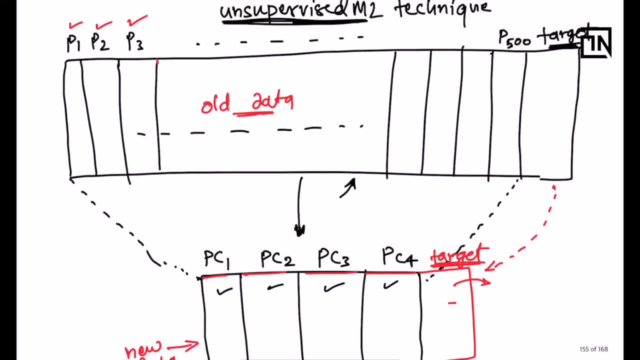 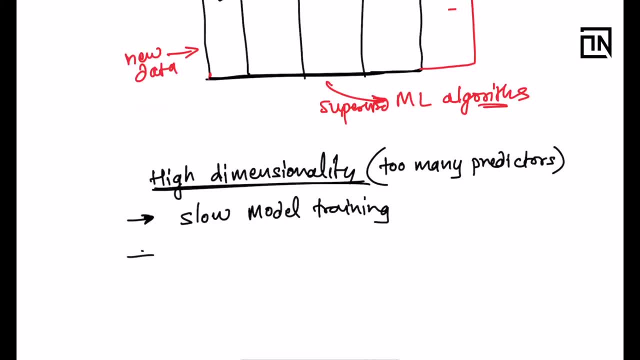 basically a compressed version of the overall data set. then you will be able to train your models very, very fast and, due to this slow model training, when your model is created, the model is also complex, which will also impact your model training. so this is a very important point. 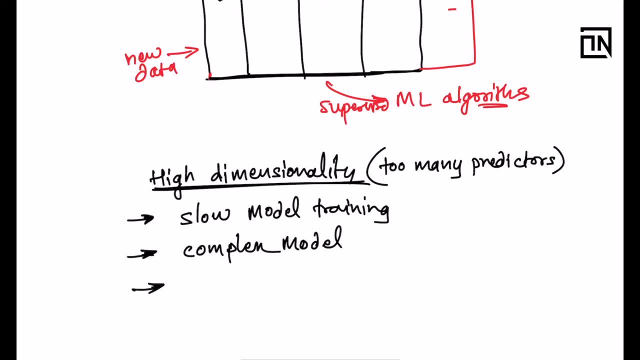 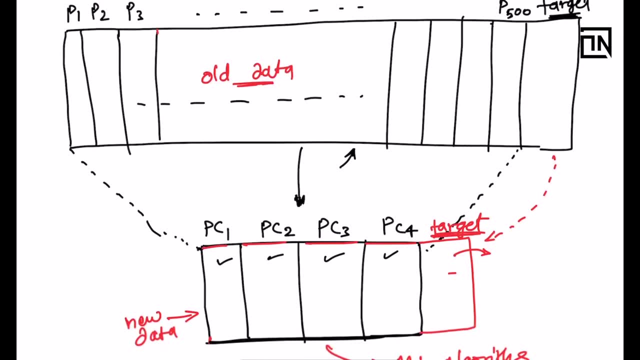 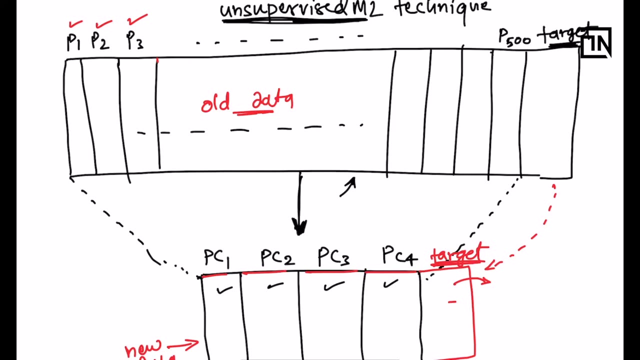 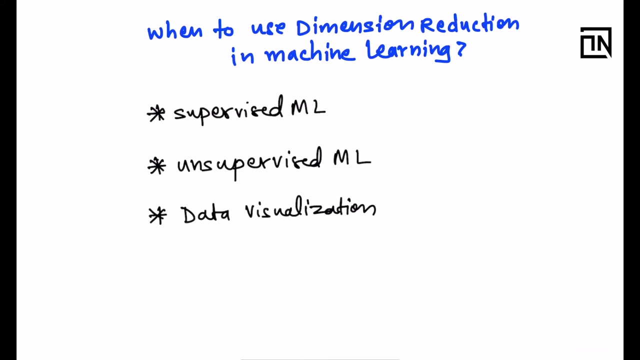 to beає hurricane 很 une super et super and super very learning and for data visualization. these are the three use cases where you can use dimension reduction, and every time the role of dimension reduction would be to reduce the number of columns so that i can do a better job, for example, in supervised machine learning. when exactly do you? 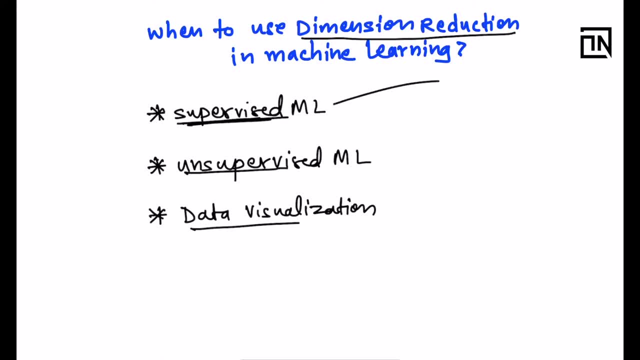 employ the dimension reduction technique. so in supervised machine learning, you have done your exploratory data analysis, you have done your correlation analysis, you have selected the feature and then you have converted the columns, the categorical columns or the string columns, into number. so often, what will happen there? there will be certain columns which have too many unique. 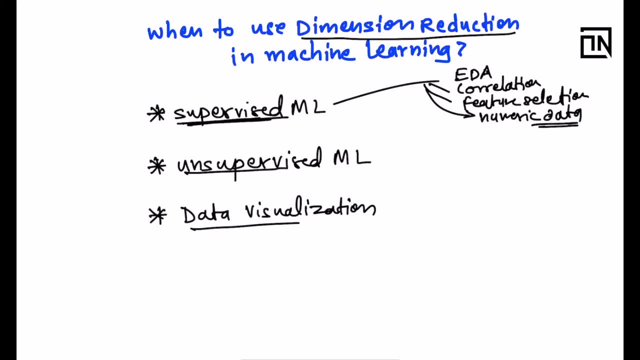 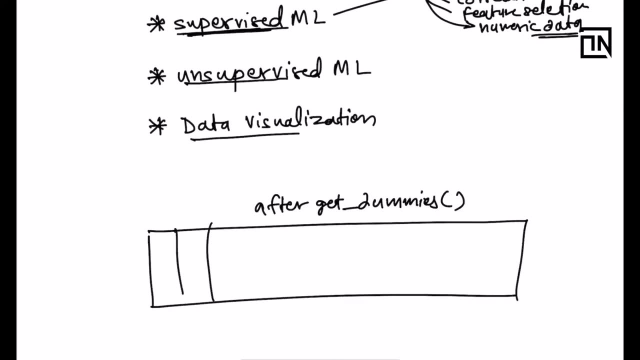 values, especially the string columns, and when you do get dummies, the number of variables will increase drastically. after you do get dummies, so when each and every unique value becomes a predictor, and then you have your target variable. so all obviously it is high diagonal, and then you have your target variable. so all obviously it is high diagonal, and then you 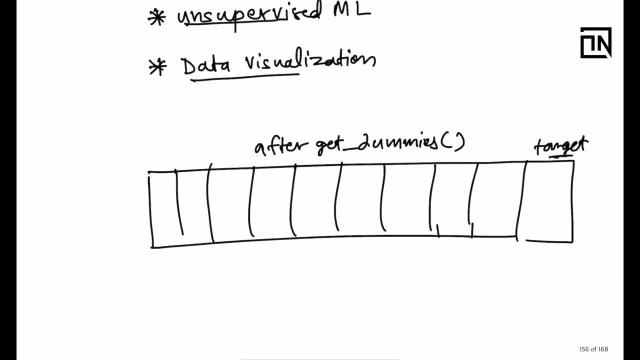 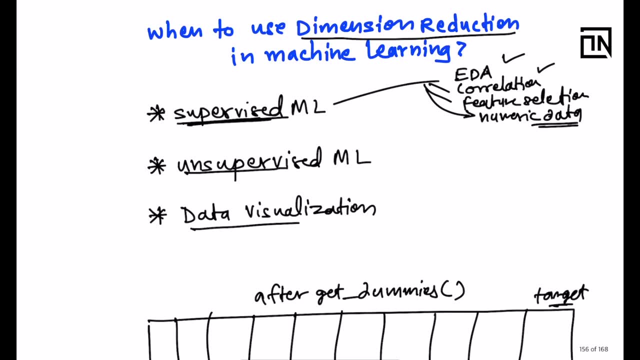 have your target variable. so all. obviously it is high dimensional and the data has inflated, so in this scenario, you can choose to shrink the predictors. so when do we perform this activity? only after all these things are done, and you are at the verge of applying machine learning, so just. 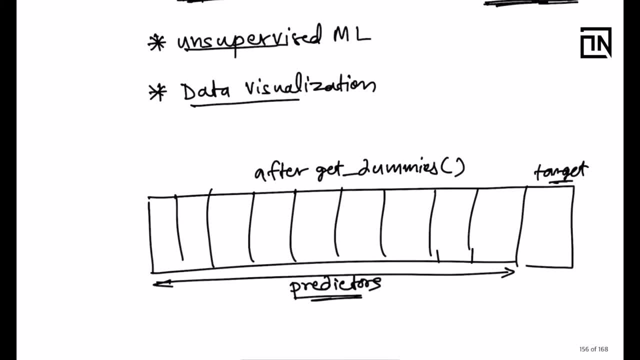 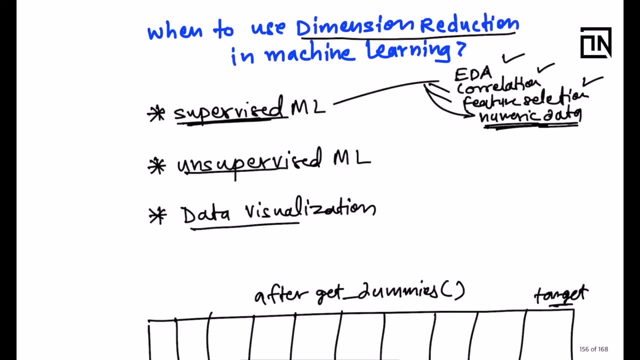 before that you take a call that there are too many predictors in the data, so let me try to represent them with smaller number of predictors. okay, using dimension reduction techniques. similarly in unsupervised machine learning. after you are done converting the data into numeric. after this, if you feel that there are too many columns and it will slow down. 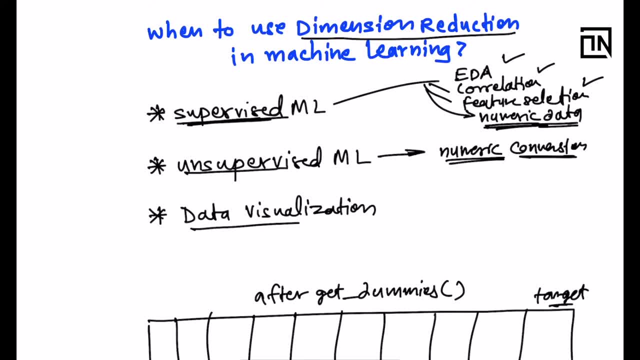 the training process of any other unsupervised machine learning, like especially clustering. let's say clustering. so in clustering, before doing clustering, you can take a call that there are too many columns. so instead of doing clustering on too many columns, let me shrink this data and do. 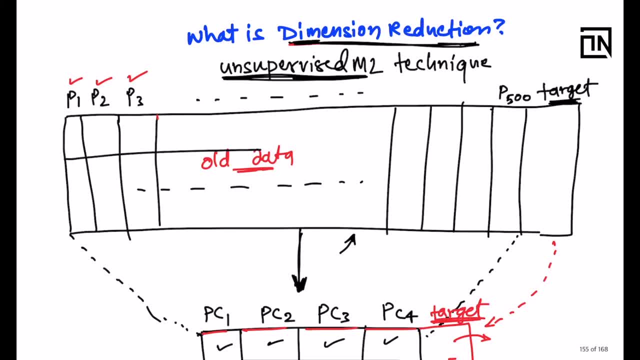 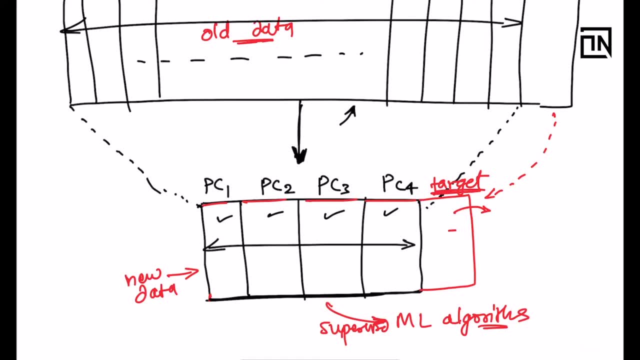 clustering on smaller set of columns. like, instead of doing clustering on all these variables, let me do the clustering only on these few variables. okay, i'm just ruling out the target variable from the picture right now. similarly for data visualization. so if your date, if your data has, 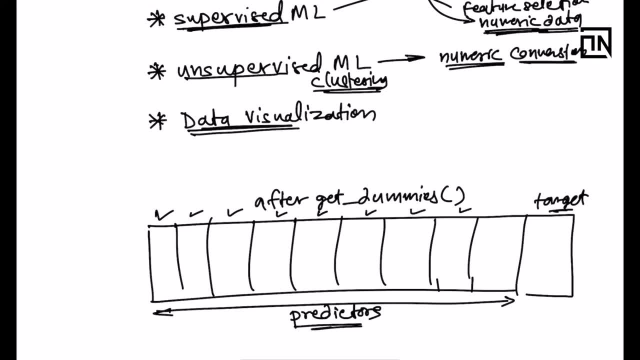 too many columns, you cannot plot the n dimensional graph for all these columns, so it will be too computationally intensive as well as hectic to code. so if you still want to, if you still want to represent the data patterns or the data variables, you can do that by using the clustering. 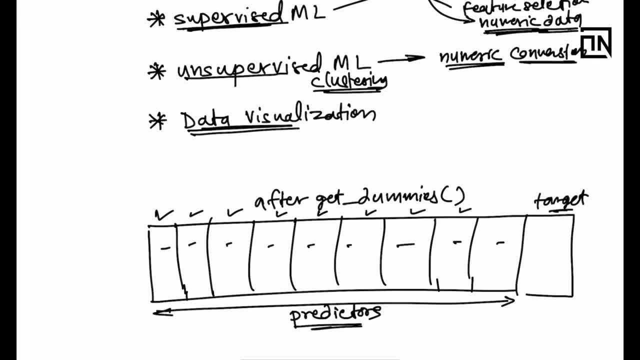 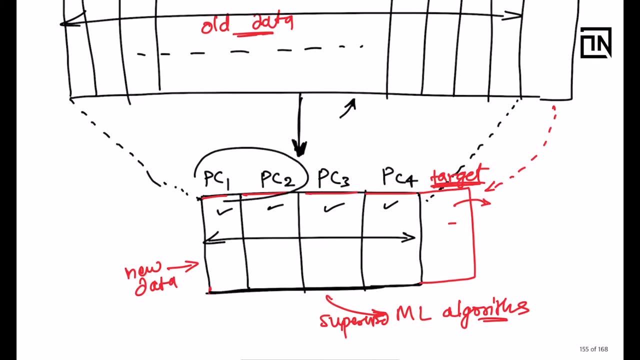 variations of all these columns, using smaller set of variables. so all you have to do is just choose the first two principal components of first two factors which are really important. okay, so instead of using, let's say, 500 columns, all you have to do is just choose these two predict, these two factors. 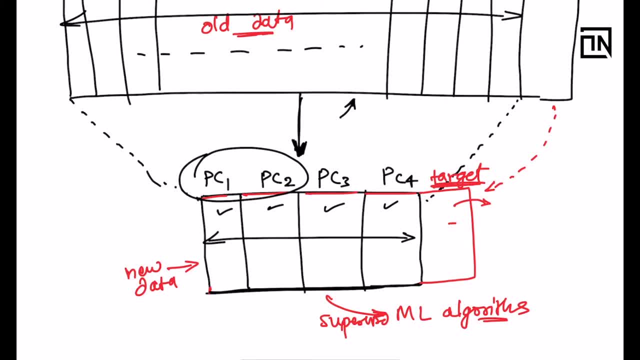 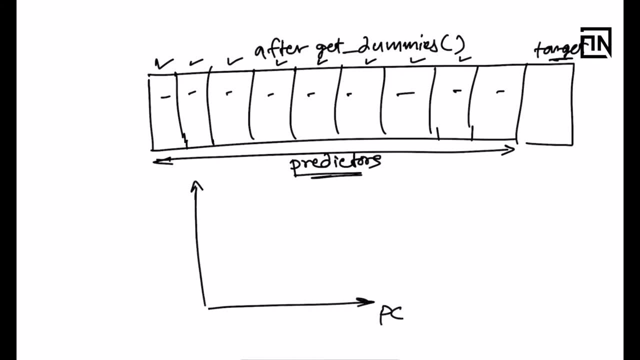 which you have just generated, or these two principal components which you have generated, and then, based on this, you can create a chart which is two-dimensional: principal component one and principal component two, let's say, for example, so data can be visualized, its grouping can be studied and clustering can be observed. okay, so when you plot a multi-dimensional, 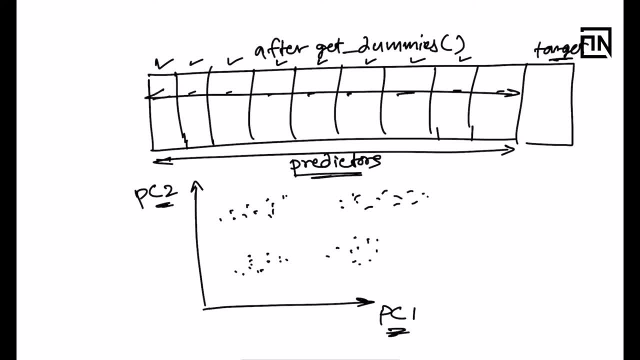 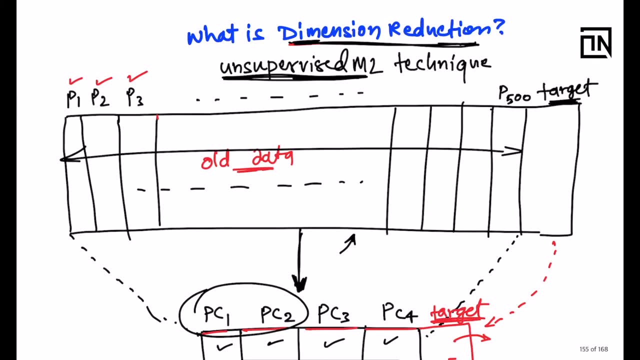 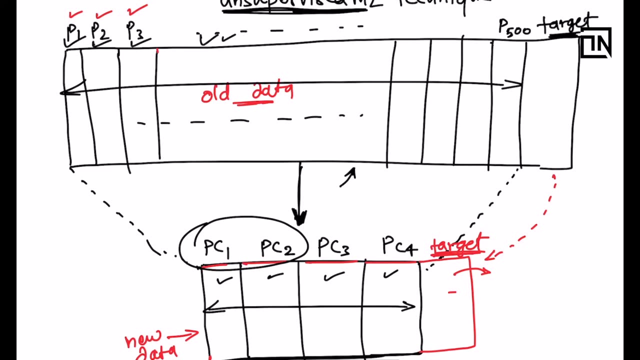 data in lower dimensions or just two dimensions. you don't just blindly choose any two columns. what you are doing is you are choosing a combination of such column because what pca, or what factor analysis, tries to do is to represent multiple such columns as a single column. okay, so there might be redundant information in multiple columns. 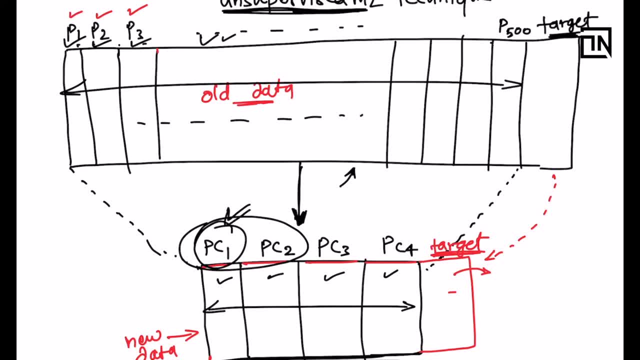 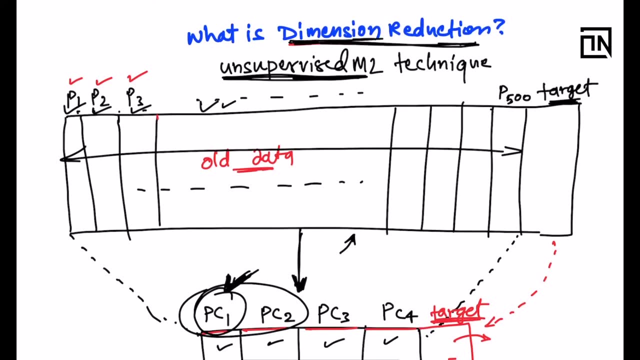 which can be clubbed together and represented as one single principal component or one simple factor. okay, so combining multiple columns together, i will get my single column or single component or single factor. this is what dimension reduction performs for you. okay, now to perform this, what are the algorithms do we have in place? 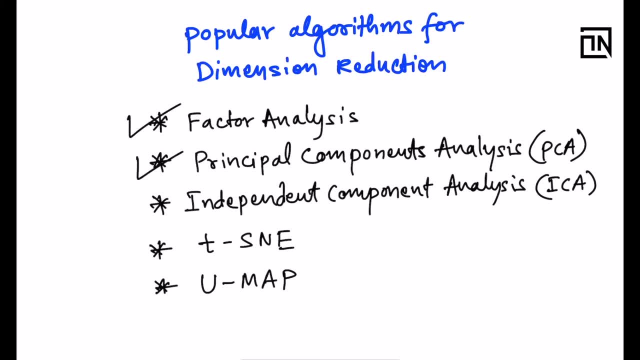 so we have algorithms like factor analysis, principal component analysis, famously known as pca, independent component analysis, or ica, the t-sne, t-stochastic neighbor embedding, and last one is umap, which is uniform, manifold approximation and projection. so these two primarily are intended towards data visualization, but can also be used for 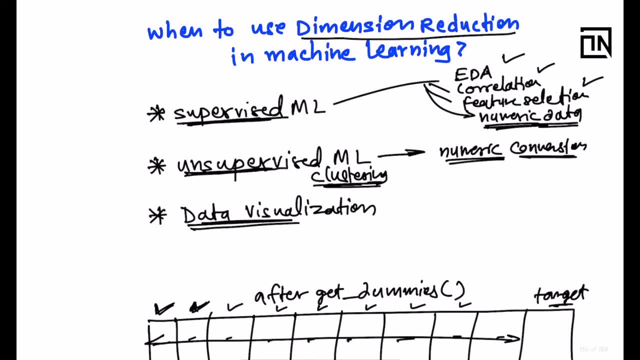 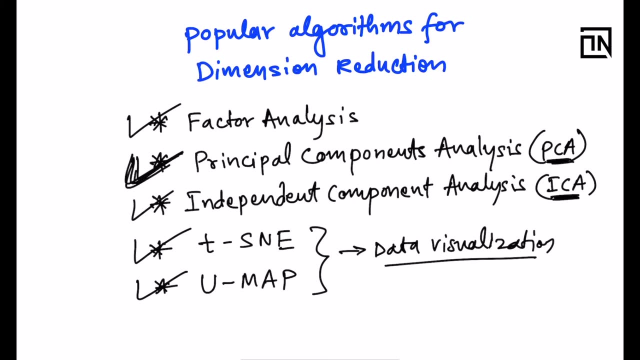 supervised machine learning and unsupervised machine learning cases like clustering or let's say some kind, some form of natural language processing you are doing before classification or regression. okay, so in those scenarios also you can use this. but the most famous of them all is principal component analysis. so now let us understand how. 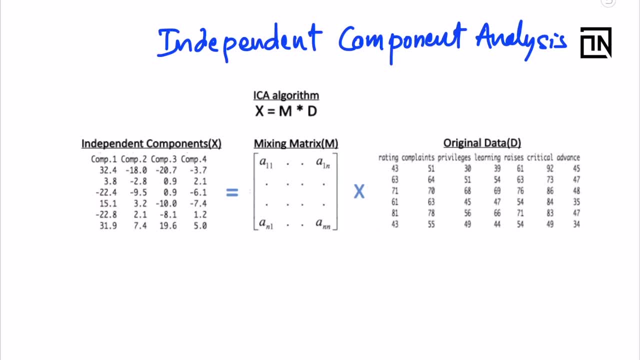 independent component analysis, or ica, works. so independent component analysis is basically trying to find independent components, components. So that name itself suggests what it is trying to do. It tries to create a mixing matrix, M, which gets multiplied with the original data in such a way that the component one 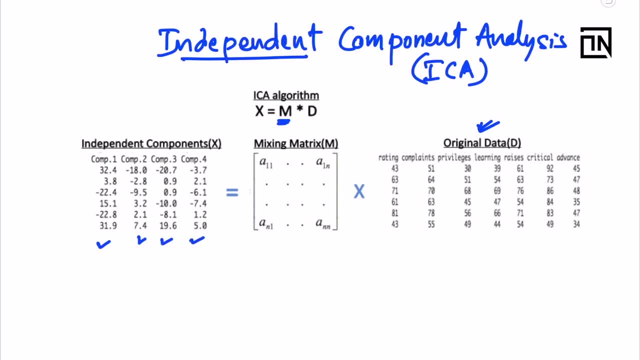 component two, component three, component four, whatever number of components you want to create, they are independent of each other. So component one is independent of component two, component two is independent of component three, But isn't this quite similar to principal component analysis? Yes, But there is a difference between correlation and dependence, Like if: 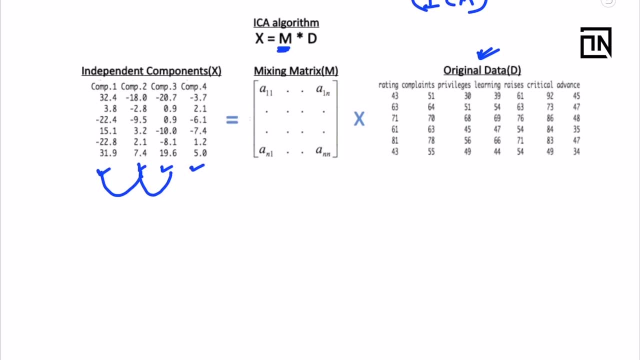 you say, if you take an example of sales, let's say if you are giving out your product with higher discounts, so you can say discounts are correlated with high product sales. You, if you offer 20% off or 30% off, obviously you will get higher sales. But if your product 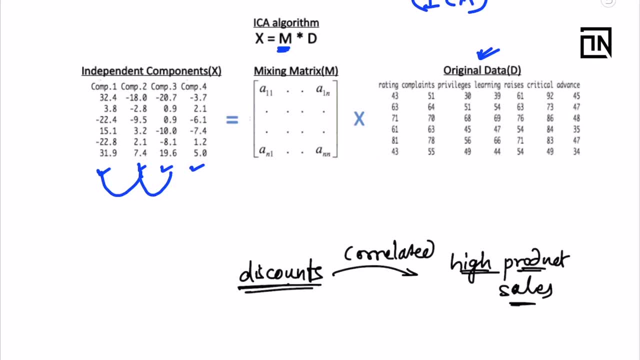 is bad. even if you try to give it at 50% off or 80% off, it won't sell. people will not purchase it. So this correlation is something which we try to see as mathematical correlation between two columns, between two vectors. Now this vector or this column is really driving. 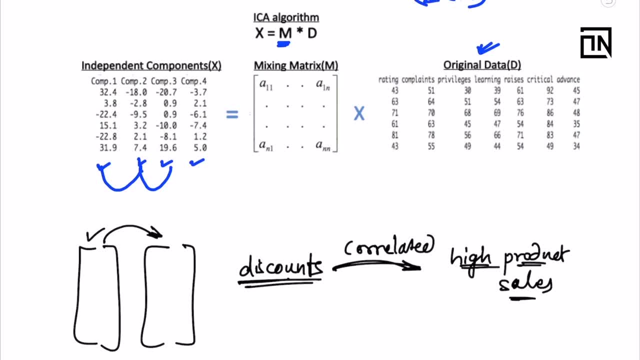 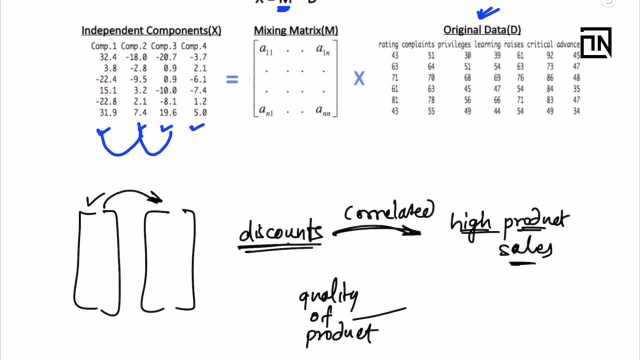 this particular another column. That is something what we say is dependency, for example, the quality of product. this quality of product is actually driving high sales. If the quality of the product is bad, no matter what kind of discounts you will give, the higher sales won't be observed. So the actual driving factor behind the scenes, 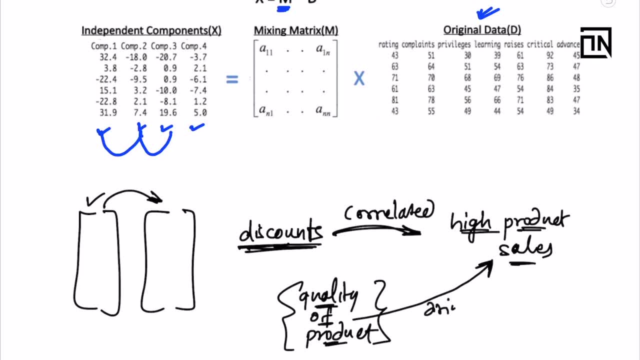 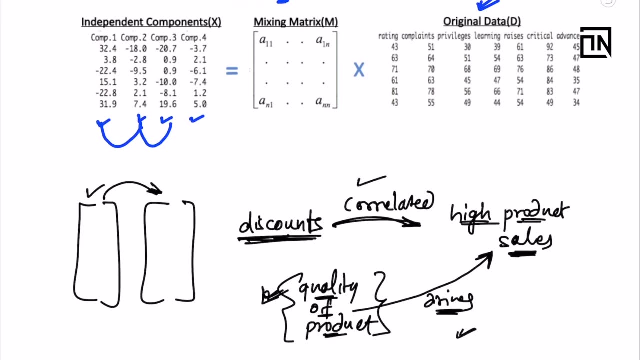 is the quality of the product. We say this drives it and that is why we say the sales are dependent on the quality of the Product, dependent on the quality. so this is the basic difference between correlation and dependence. dependence has to do something with causation and correlation is just mathematical relationship. 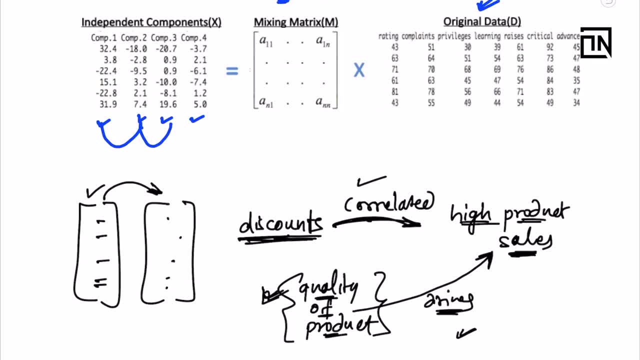 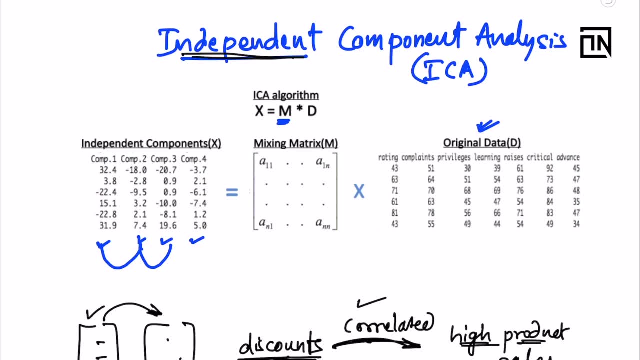 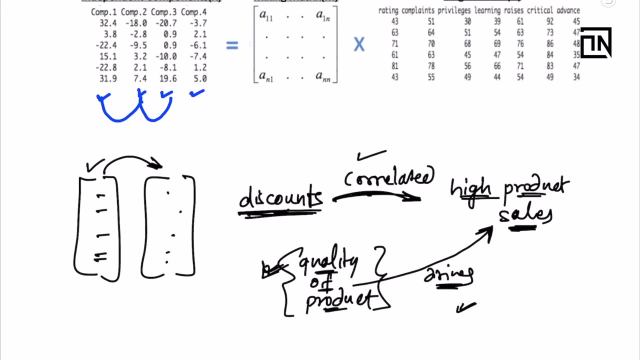 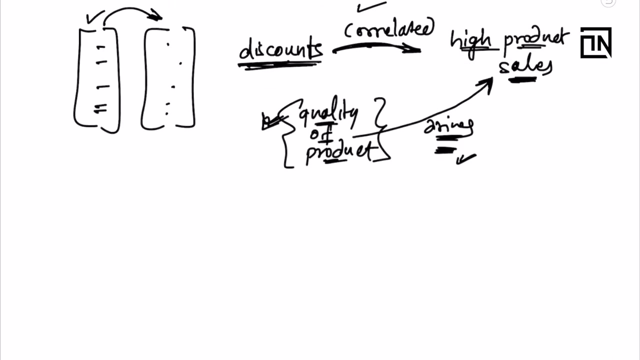 between two vectors, they might not really cause each other to vary. okay, so independent component analysis is the journey to find out such components which are totally independent from each other. and we are not talking about correlation, we are talking about independence, and this is the core difference between principal component analysis and independent component analysis. pca tries to 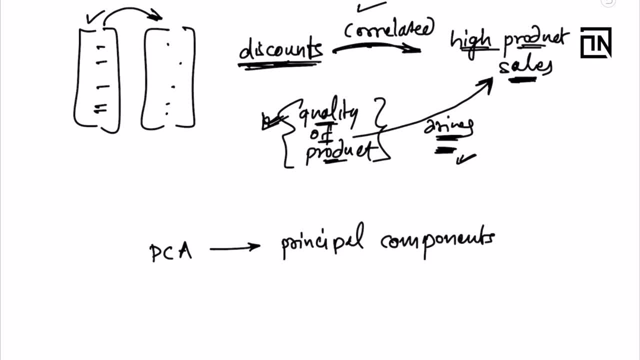 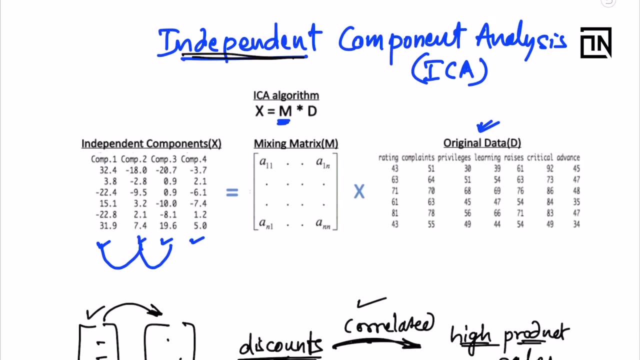 find certain principal components which are not correlated with each other, and independent component analysis tries to find the components which are not dependent on each other, basically independent from each other. so here the causation is a driving factor. now, in order to find out such kind of values, we